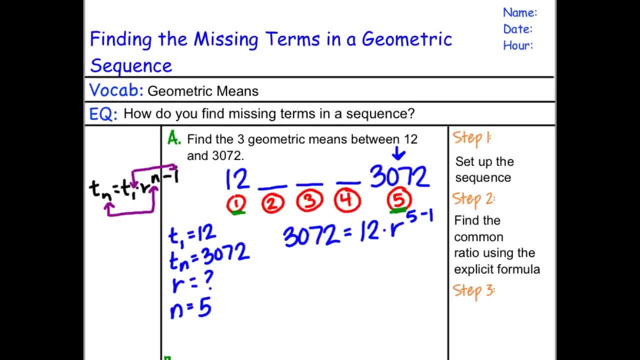 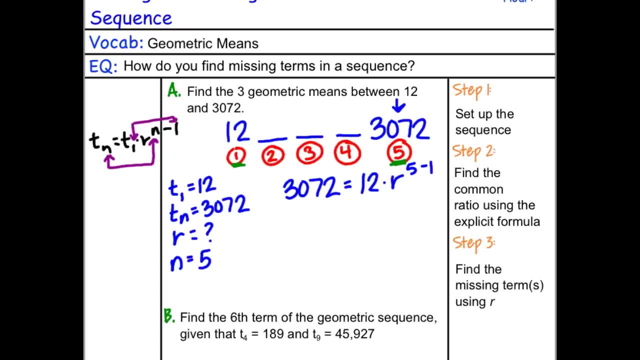 numbers that were given and subtract them. Then, once we've done that, we find our missing terms. So first we have to solve this. I'm going to rewrite this first. We have 3,072 equals 12 times r to the fourth, because 5 minus 1 is 4.. So we will divide both sides. 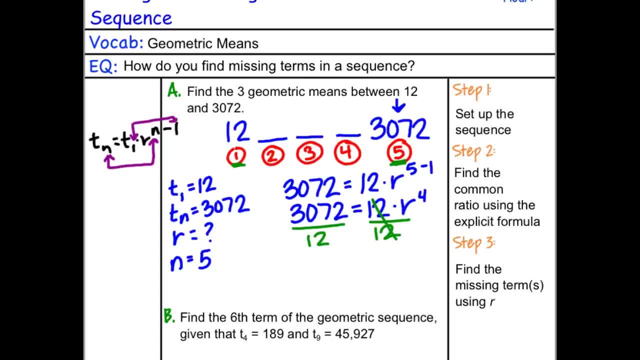 by 12. And that gives us 256 equals r to the fourth. Now, if you recall, to undo squaring, we square root. So to undo a fourth power, we're going to take the fourth root. Some of you are probably going: whoa, whoa, whoa, whoa, whoa. 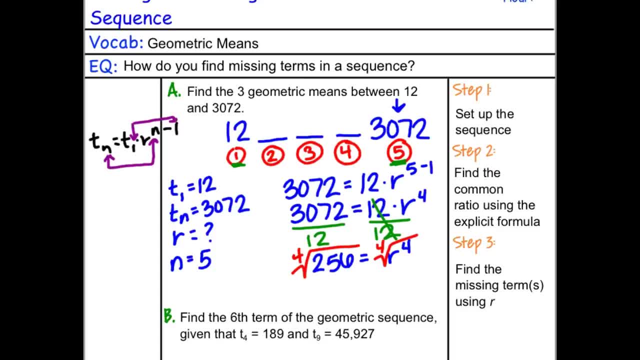 I have no idea how to do that by hand and I don't know where to get it on the calculator. Now. if you have a standard TI-30X2S- non-graphing but scientific calculator, you will see above the caret key you'll see a y square root of x or a blank square root of x. 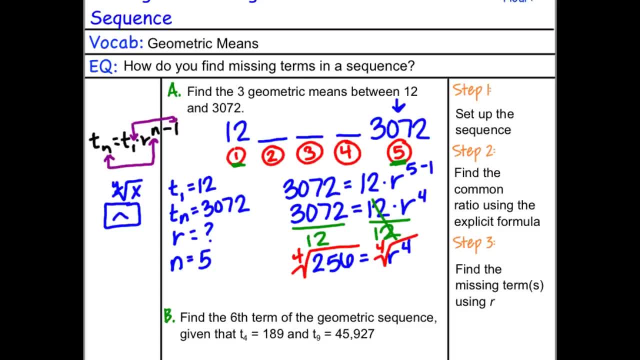 That's trying to say your power. So what you'll do for that is you will hit the four, Then you will go second and hit, Hit the caret key and then you will type in your 256.. Now, if you have a graphing calculator, you'll hit the four. 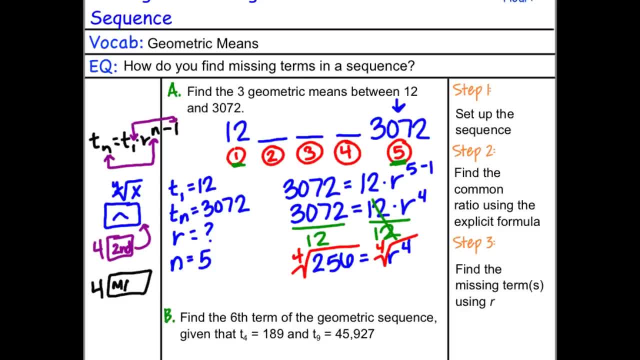 and then you will go to the math button and then that's option five. It'll look like this: It'll have a little box with a square root or a radical x. So when I do that, I end up getting that r equals four. 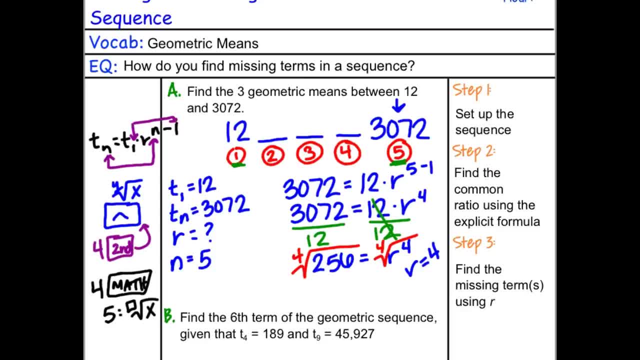 because four times four times four times four is 256.. From there I take each of my numbers and I multiply by four. Twelve times four is 48.. 48 times four is 192.. 192 times four is 768.. 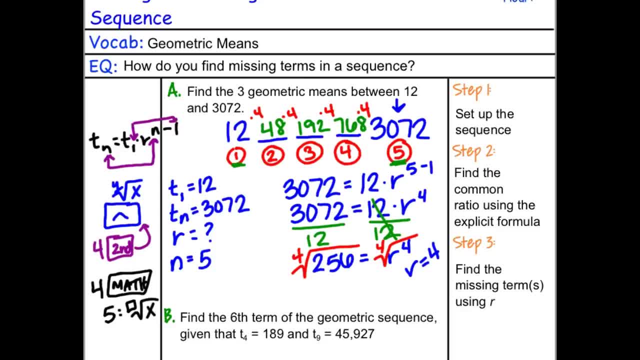 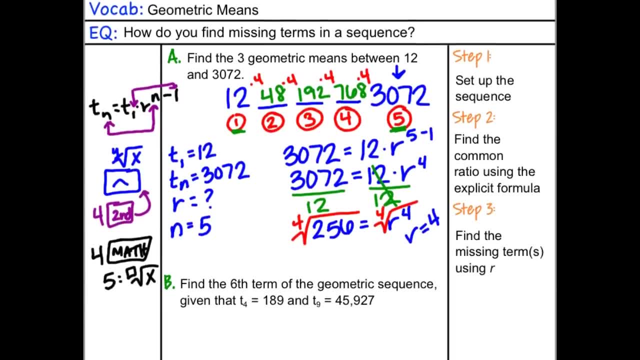 And then just to check to make sure I did it right, it took 768 times four and got 3072.. The second type of problem you're going to see is one like B, where it says we're given the fourth term and the ninth term. 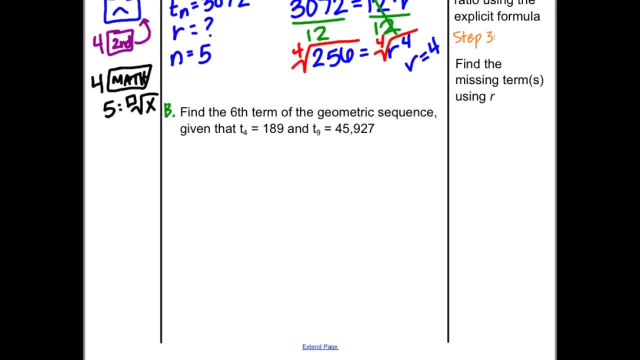 I want you to find the sixth term. So we start by setting it up in a similar fashion: We're given term four, and then I'm going to put five term, six, term seven, Term eight, and then we're given term nine. 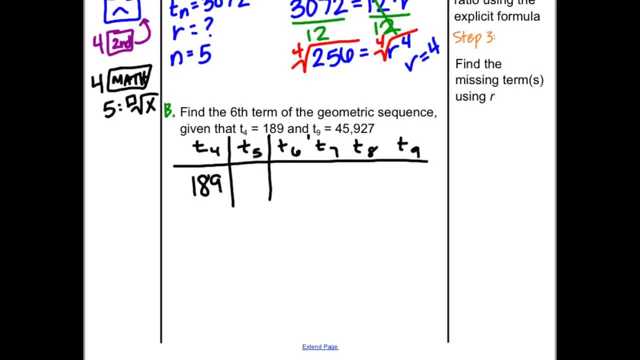 Term four is 189.. Term six is what we're trying to find, And term nine is 45,927.. So, same idea: We take our ending term. This is our term n, This is our pseudo term one. So we take what we end with. 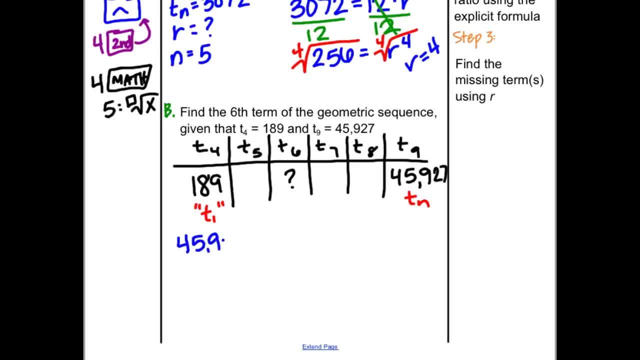 Our 45,927, and that equals the first term we're given, 189, times r that we don't know. Now. 45,927 is term nine and 189 is term four. So we use nine minus four instead of. 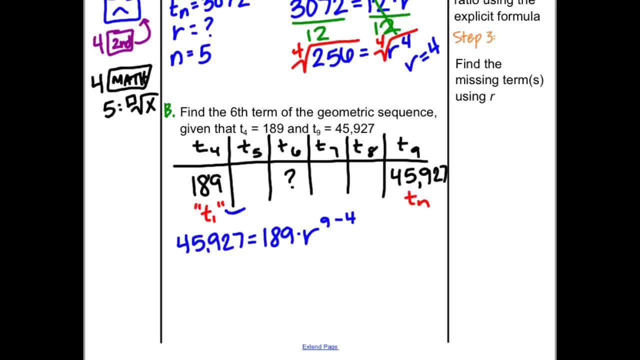 otherwise, you could look at it as you apply the common ratio one, two, three, four, five. Well, ironically, nine minus four is five. So then we simplify: We got 45,000, oops, not 49,000,- 45,927. 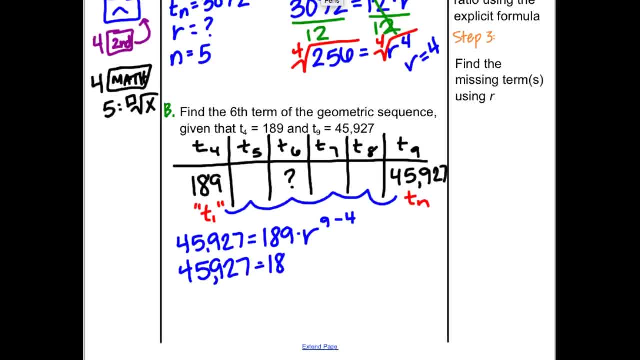 equals 189 times r to the fifth. We divide both sides by 189, and we get 243, equals r to the fifth. Before we had an r to the fourth, so we took the fourth root. Now we have a fifth power. 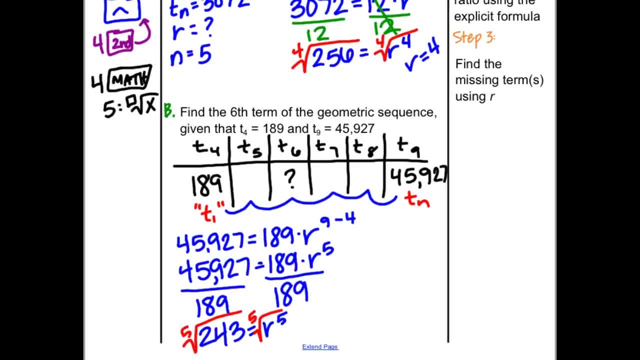 so we're taking the fifth root And it works the same way, except now, instead of typing in a four, like I told you to do before, you'll type in a five before you hit the special button, And when I do that, I get r, our common ratio.